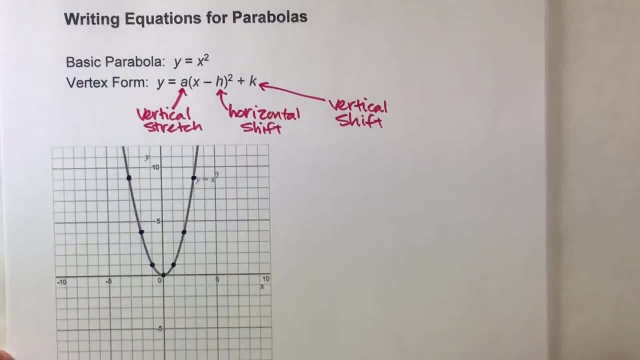 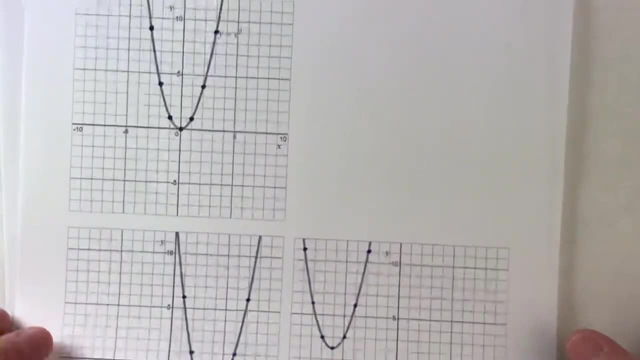 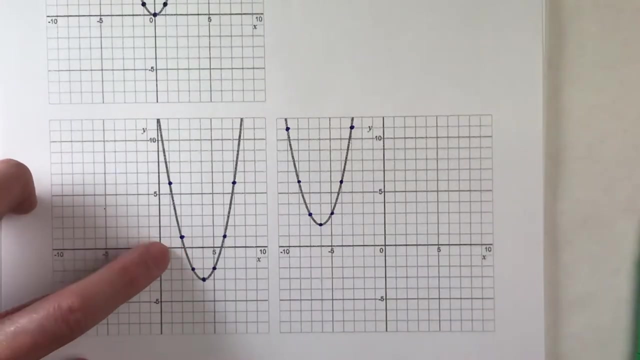 then this is going to be negative, Alright, so there's basically three things we're looking for when we're writing these equations. So let's do a couple of examples, Alright, so we'll start with this one right here. Now notice: this one is basically the exact same shape and size of a normal parabola. 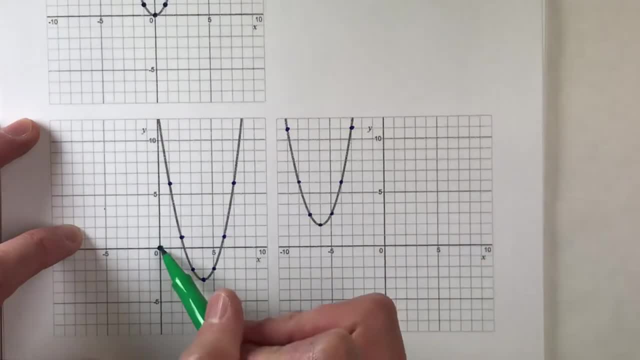 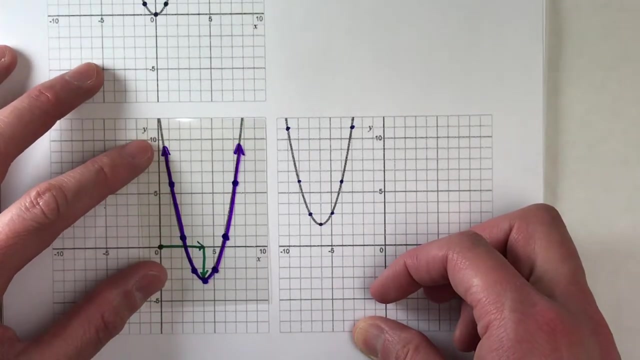 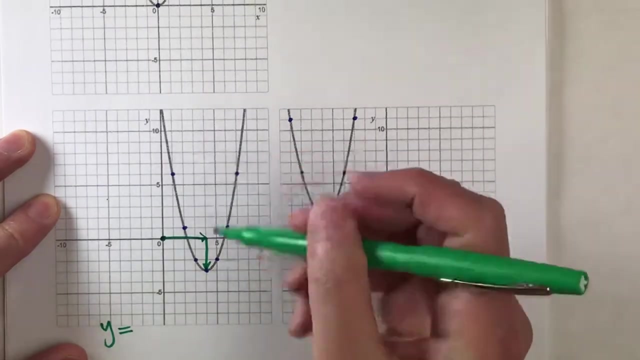 except, instead of the vertex being at 00, it's been slid over to the right four steps and then down Three. Alright, so if you imagine, here's our basic parabola. We've just shifted it over and down And now we have the exact same parabola. So for our equation y equals, we know there's no vertical. 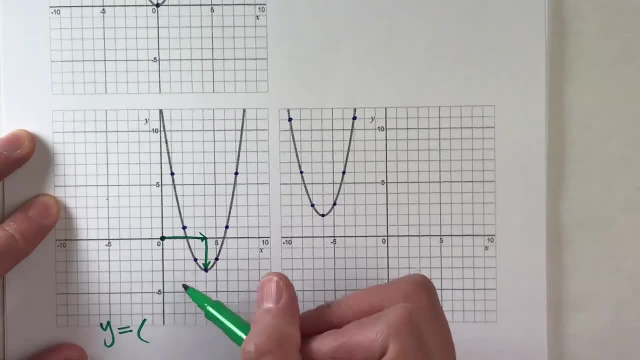 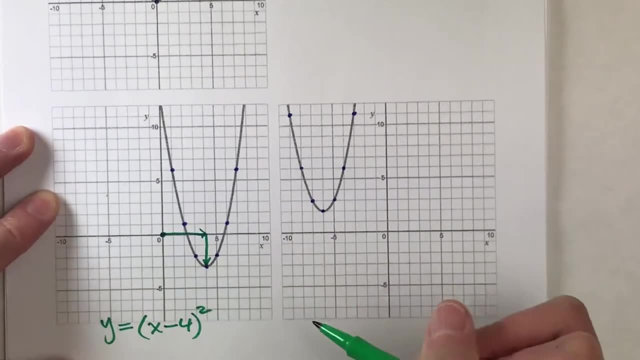 stretch, so we don't have to worry about a number in front of the parentheses. But we're shifting it to the right four units. So we're going to do x minus four squared. Now we're also shifting it down three, so that the vinegar will be higher than or equal to our kilogram. harder and harder. 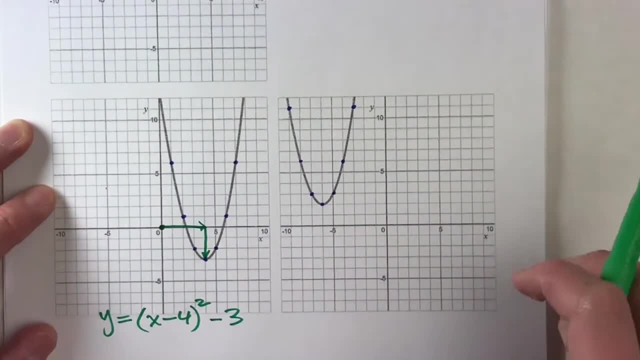 but what we're going to do here is take our algebra and the unit and we'll just practice. when we're sleeve, The cameras are not going to get fell in because their number's going to need to find the properties. so end of this equation. we're going to minus 3.. There's your equation. Alright, Let's do. 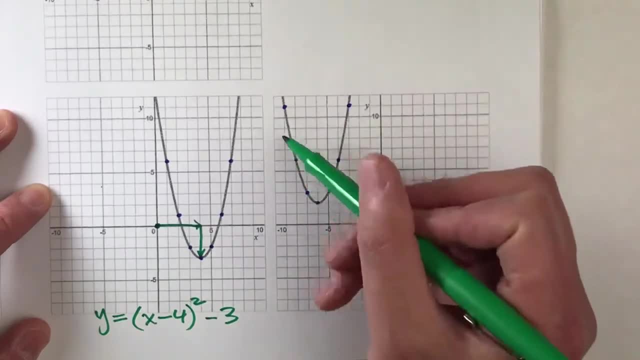 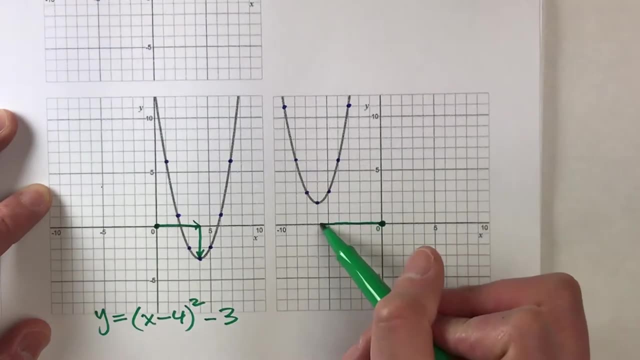 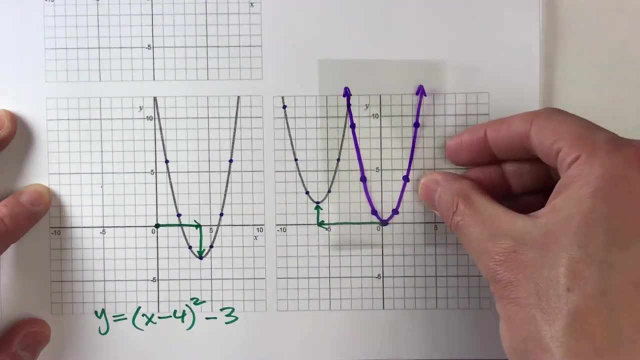 another one, This one right here. Again, it looks like the same shape and size as the original parabola, except instead of having the vertex at the origin, we've shifted to the left 6 units and then up 2.. Alright, So you imagine here's your basic parabola. We've 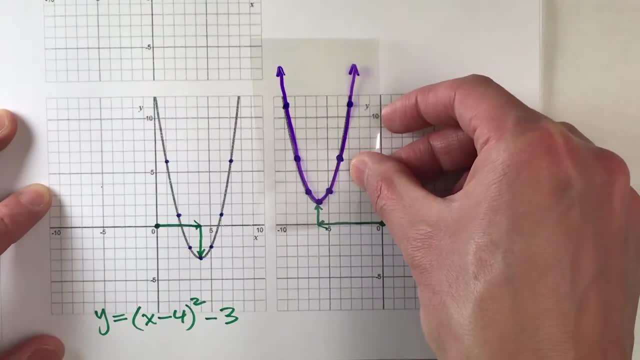 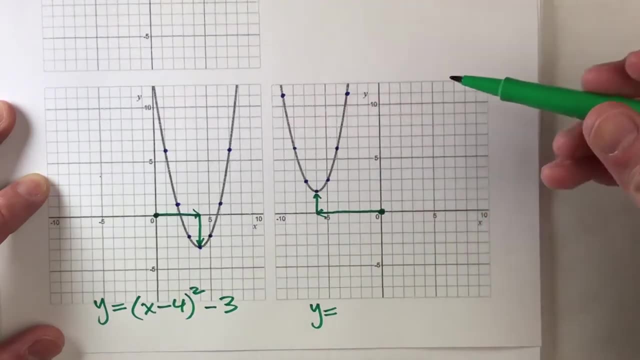 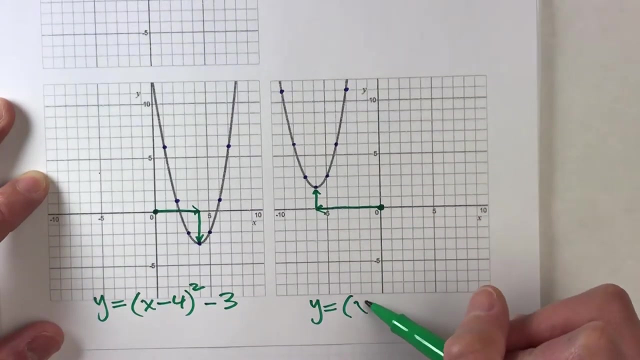 shifted it over and up and there it is. So let's write our equation: Y equals. now remember, it isn't vertically stretched at all, so we don't need a number in front of the parentheses. but we did move it to the left, 6 units. So we are going to add 6 to x inside the parentheses. 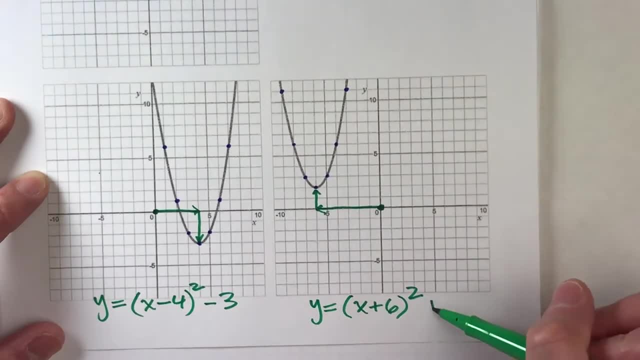 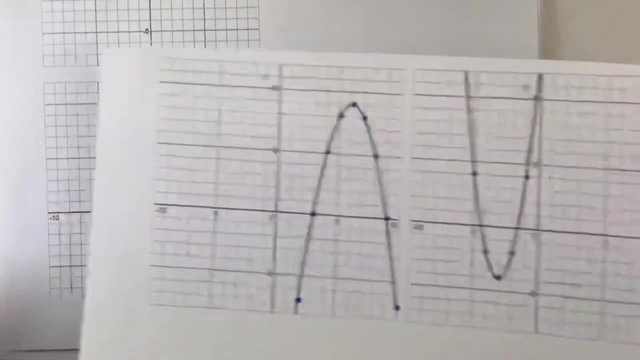 And then also we shifted it up 2 units. so at the end of the equation I'm going to put a plus 2.. And there's my equation for the parabola. Alright, Let's do 2 more. Here we go. Now. this one's an interesting one, So notice. 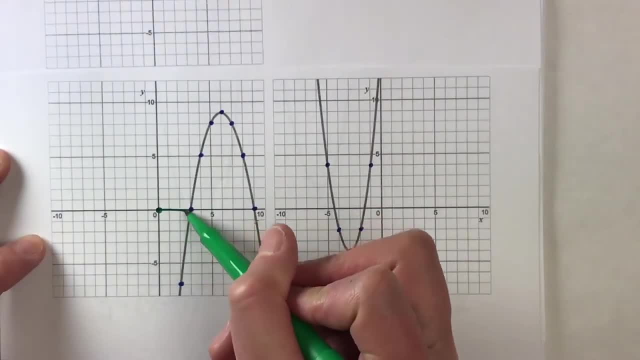 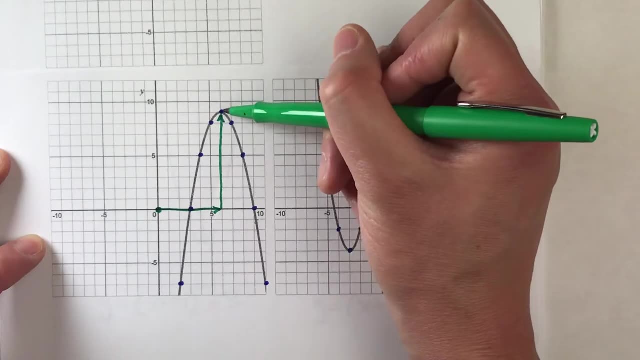 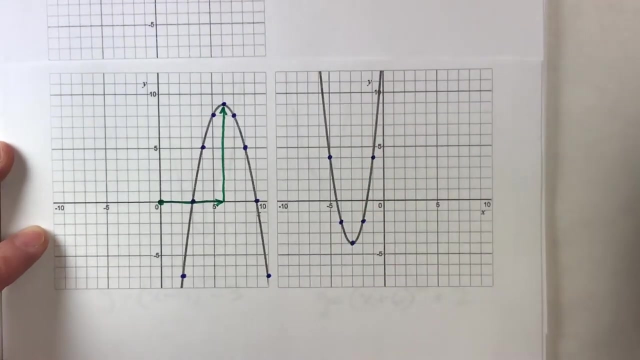 the vertex normally starts at 0, 0, but we've shifted it to the right 6 units, and then we've shifted it up 9 units, But then also notice it's also flipped upside down, So we've got all 3 things going on here. 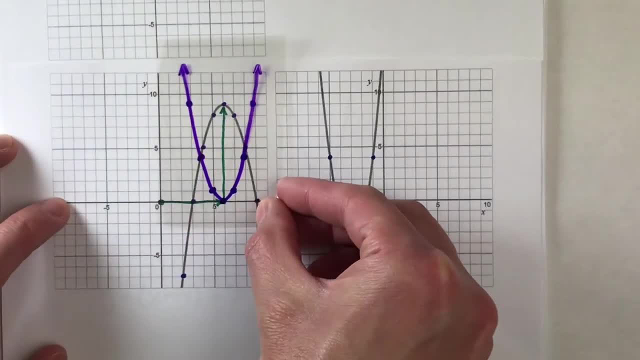 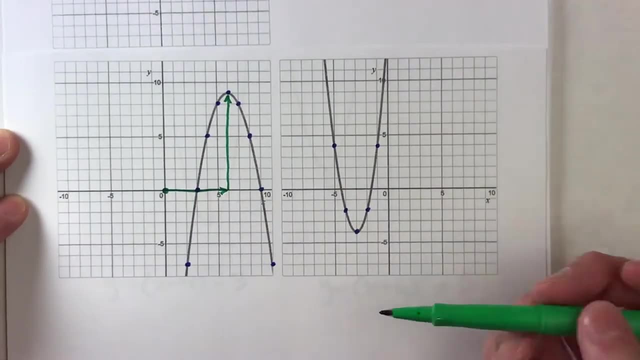 So we've taken the parabola Subtitles by the Amaraorg community, We've shifted it, We've shifted it And we've flipped it upside down, So we're going to have to pay attention to all those things today. One thing, though: notice that we didn't. 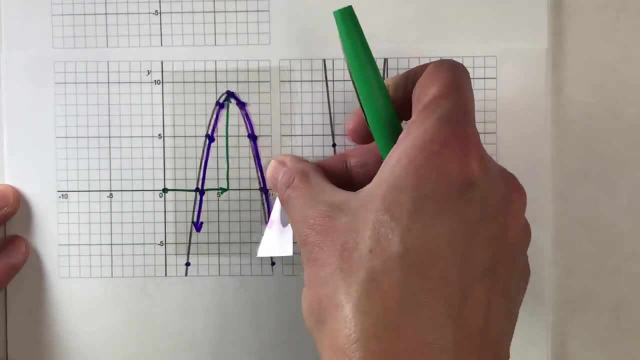 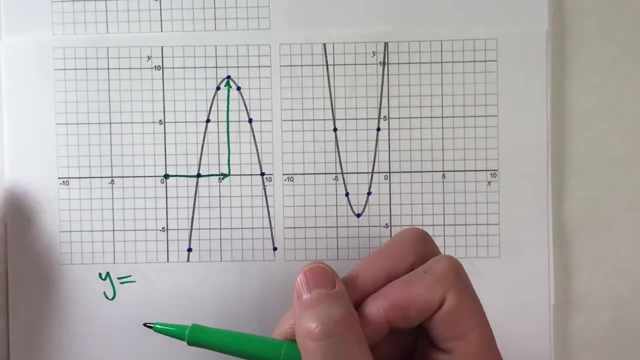 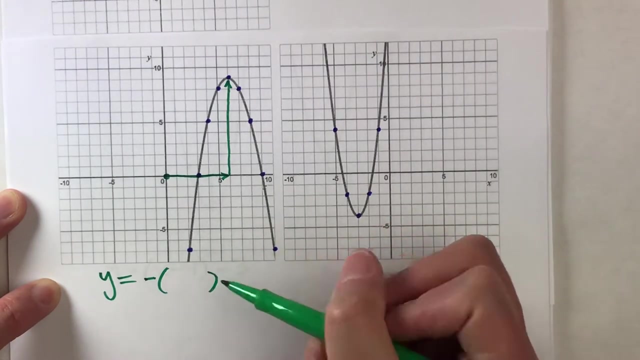 stretch it, It's still the same size as the original parabola. It's only flipped upside down, So my equation's going to be y equals. now, like I said, it's not stretched, It's only flipped upside down, So I'm just going to make this a negative parentheses. Alright. 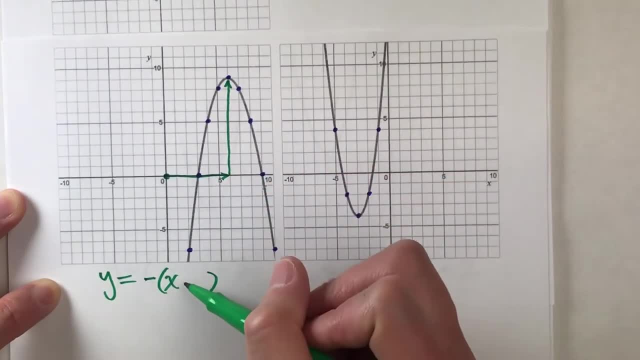 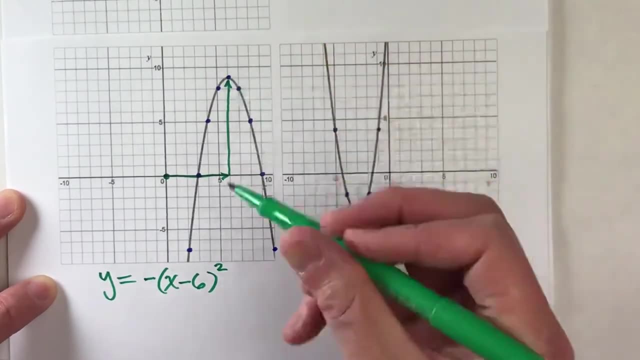 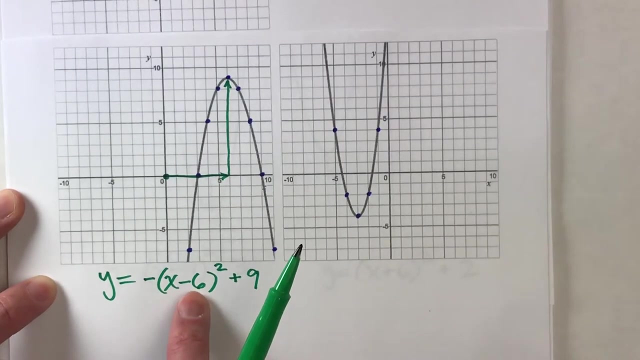 Now it's moved to the right 6 units. so I'm going to do x minus 6 inside the parentheses before I square it, And it's shifted up 9 units, So at the end it's the equation plus 9.. And there is my equation. Notice: this shows that it moves over to the right 6.. This 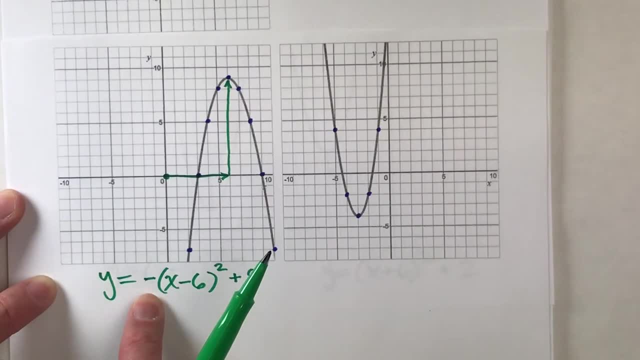 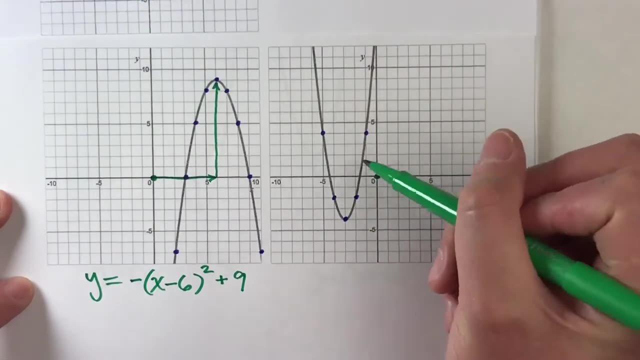 says it moves up 9. This says it's flipped upside down. Alright, Last one, Now this one. notice the vertex usually starts here, But notice the vertex usually starts here, But, but it's been shifted over to the left. three. 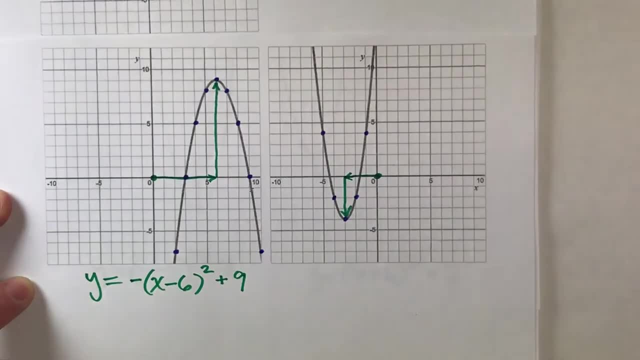 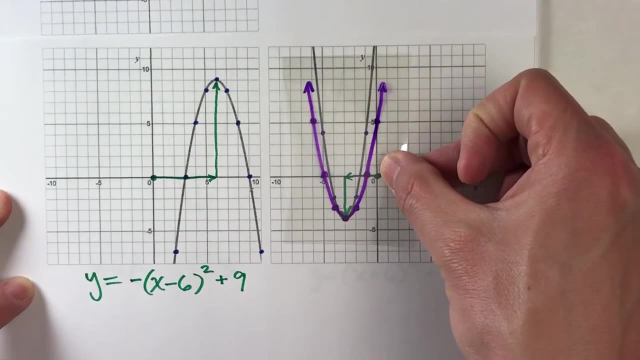 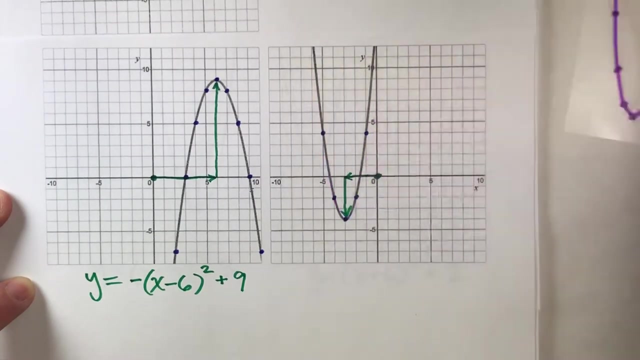 and then down four. all right, But there's one more thing you have to pay attention to on this one. See, if I move this three and down four, notice the parabola's different shaped than the original basic parabola. all right, 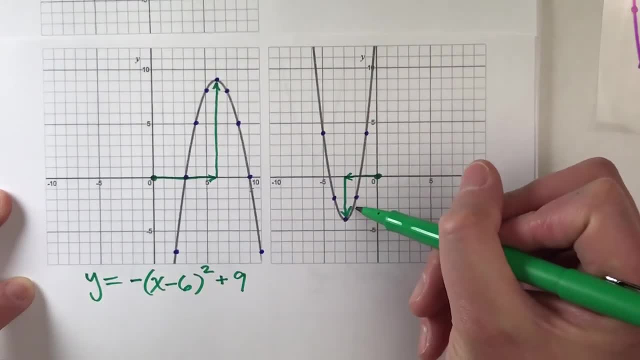 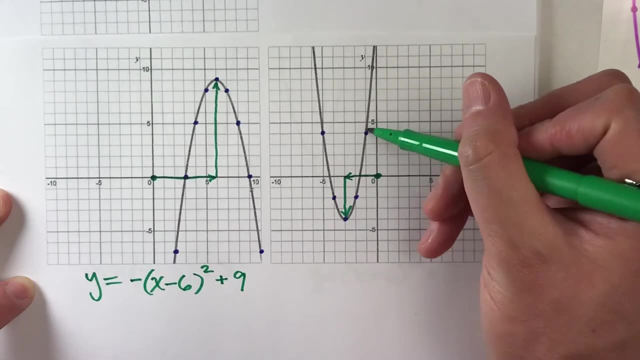 So, instead of from the vertex, the next point being over one up one, this parabola's over one up two. And instead of over one up three, for the next point, it's over one up six. This one's been stretched vertically by a factor of two. 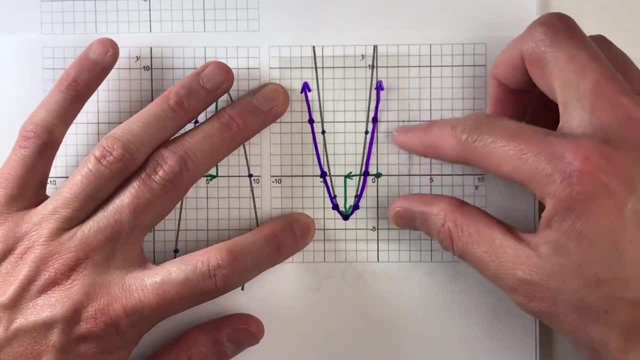 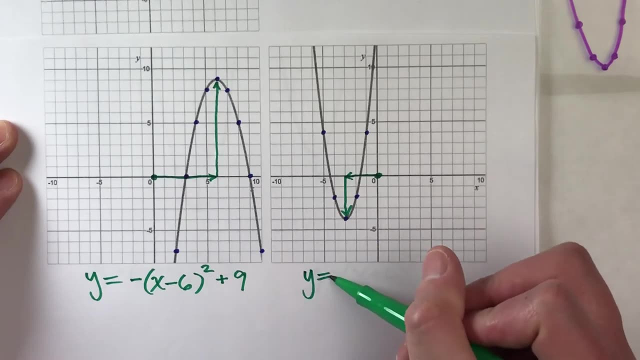 And that's why it's taller and skinnier than the basic one. So this one actually has a vertical stretch of two. So that's gonna come into play in our equation: Y equals, like we just said, it has a stretch of two.